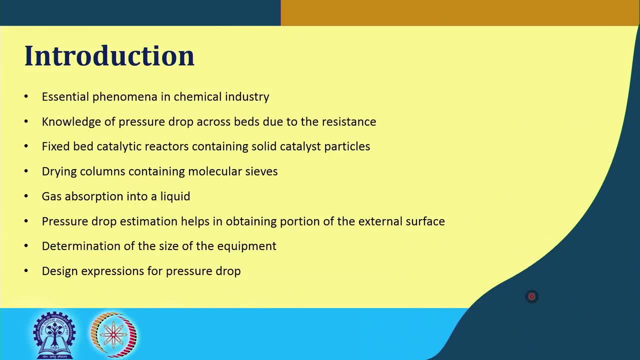 as I said, the solid particles can be of a bigger size, or, let us say, the fine particles. Essentially, we have to. our goal in this section is to understand how we measure the pressure drop across the bed, because that is one of the vital component for designing equipment. that. 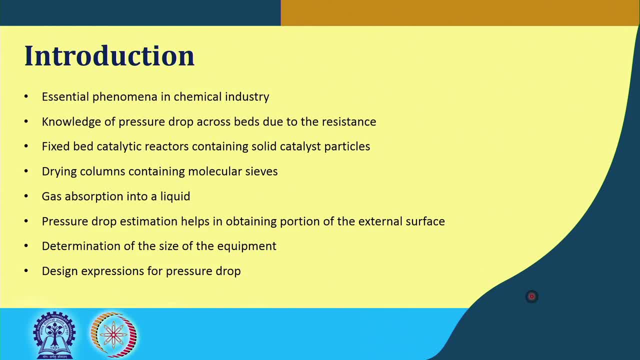 handles such operation. ok. So the examples: one of the examples that I gave I have given was a fixed bed catalytic reactor. let us say where SO 2 is converted to SO 3. in presence of solid catalyst bed, There can be the drying column that consists of molecular sieves through 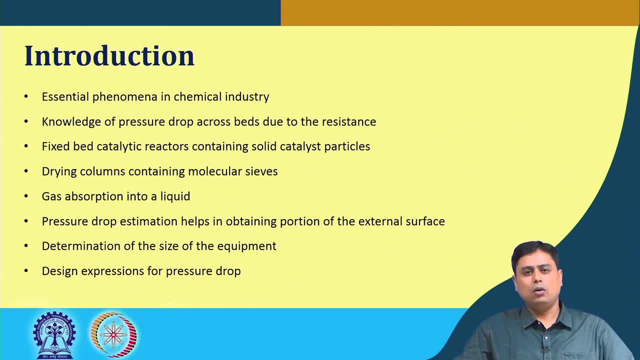 which the fluid is flowing, ok, When there is gas absorption into liquid. where the liquid is liquid, flow is happening from top to bottom and the gas phase is blown from the bottom to the top. So this absorption depends on the surface area available. ok, Now this pressure. 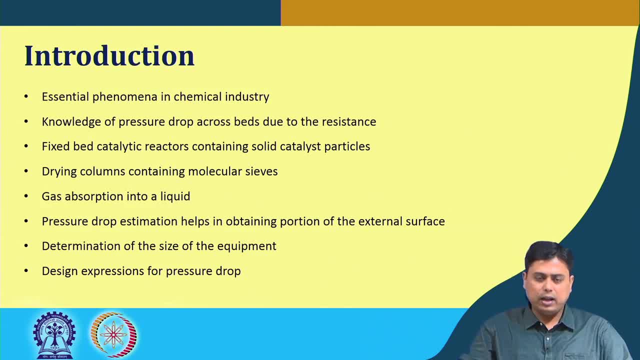 drop estimation helps us to give an idea that how much is this available external surface on which this several. let us say, in case of solid catalyst, that the reaction can happen. on the solid surfaces, the adsorption can happen And this solid surface basically dictates. 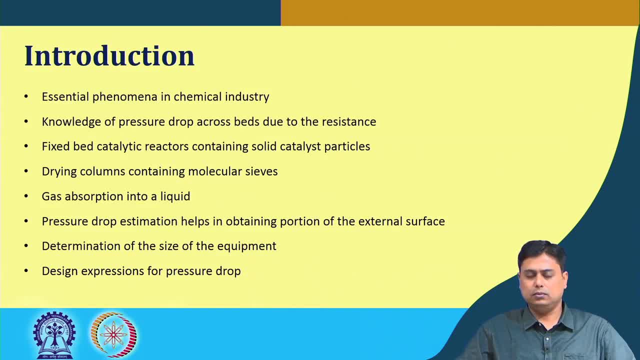 that how much resistance will be there, as well the available surface area. So in determining the size of the equipment or designing of this equipment, that expression for pressure drop is very essential. Now the point is that in several, in most of the industries, this flow through this such packed beds. 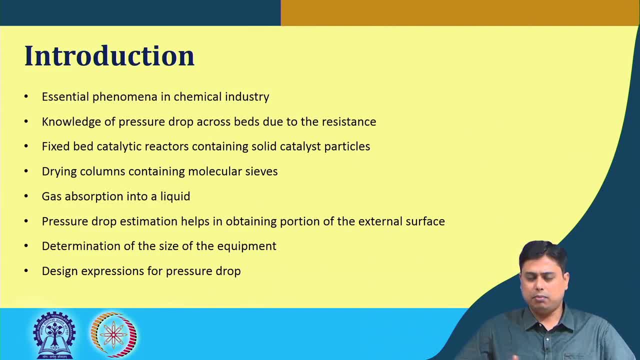 Or the granular beds or let us say, the powders, is not of a single phase flow. ok, There are multi phase. multi phase flows happen in those cases. but for the time being we will focus at first at the single phase flow. when it 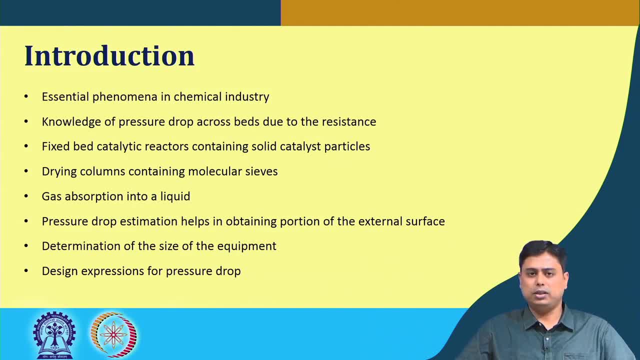 happens through such a bed of the material of several different object of different size that can be of different densities. ok, So the essential goal in this section is to understand that how the pressure drop will vary when a fluid flows through a stack of. 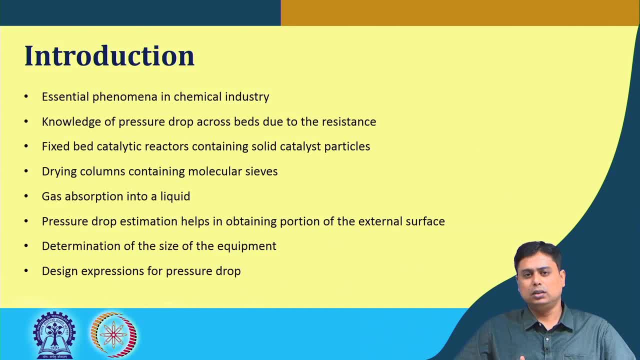 particle or a bed of particles, bed of powders, particles having different sizes, particles of different shapes and similar things. So the point here is that if the fluid flow through such a stack of particles, as something areء, but when the fluid flow through a bin, from in to a particular bond, So at the end you will see what the normalized peak it, because like that it stays welcome. it belongs there in another nei, but still hasn't discovered. So the point here is that where does embroidery Karere in which a bunch of these particles can be cultivated, filling discussed? 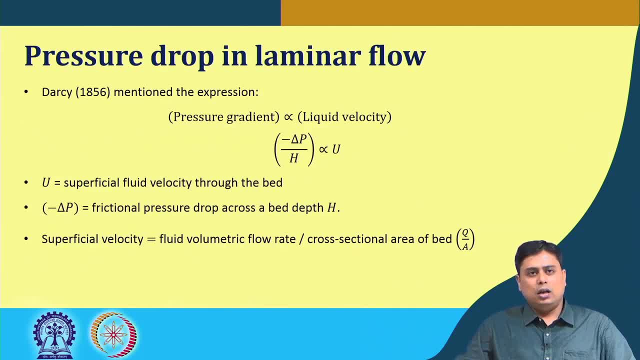 So the point here is that in 1856, Darcy initially proposed an expression when he did the experiment of a fluid flowing through a bed of sand- water flowing through a bed of sand. Observe that the pressure gradient is basically proportional to the velocity of the fluid, which means: 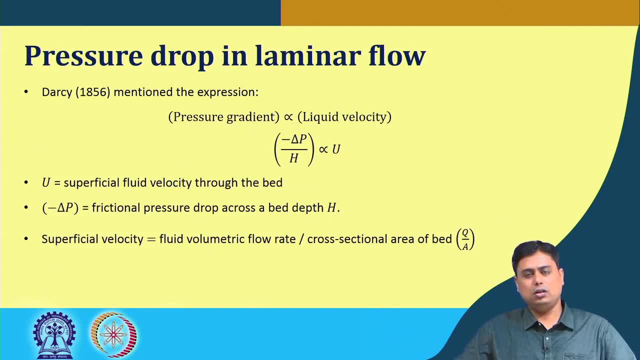 the pressure gradient here is the del. p by h is proportional to the liquid velocity, where u we define as the superficial velocity that is happening through the bed. ok, So why the negative sign? You already know this thing, that here the flow is happening from high pressure region to the low pressure region. ok, So the point here, this frictional, 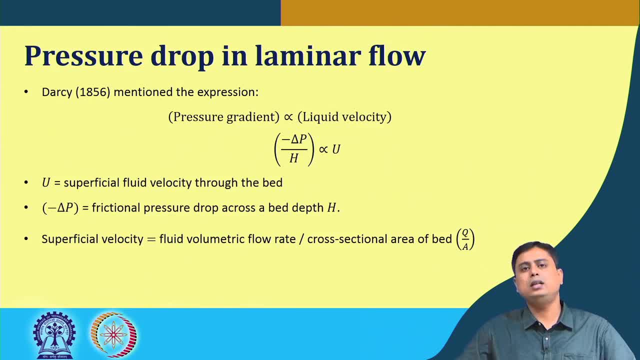 pressure drop. So this is the frictional pressure drop. So the point here, this frictional pressure drop across the bed having a height or depth, whatever you say. if that is h, then this del p by h is basically proportional to the superficial velocity, where the superficial 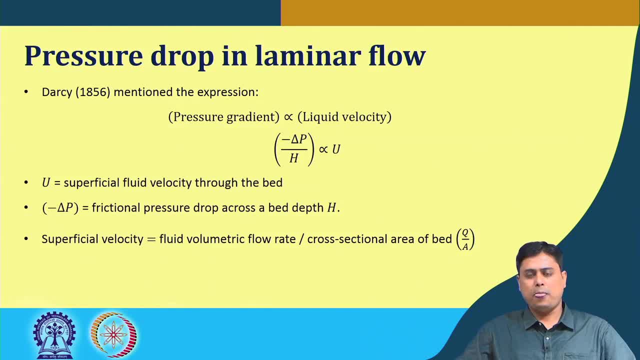 velocity is nothing but the fluid volumetric flow rate per unit cross section of the bed. So if you have a q unit of volumetric flow rate happening through a cross sectional area of a unit square and q is your volumetric flow rate, that is, unit q per minute hour or. 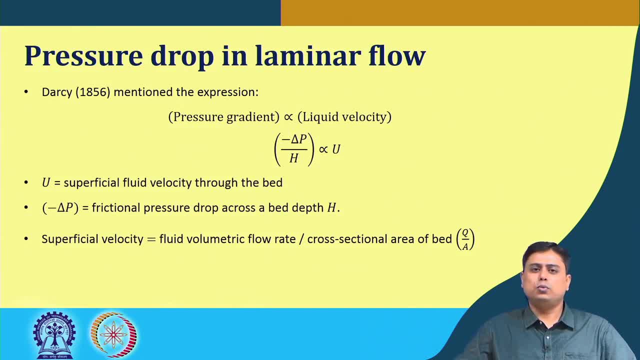 time, then q by a is basically the superficial velocity. ok, Now the thing is that this stack of material or the bed of powder object, whatever you say, when it is packed, if it is not a sequential, sequentially packed- ok, we call this- is that would be a random packing. 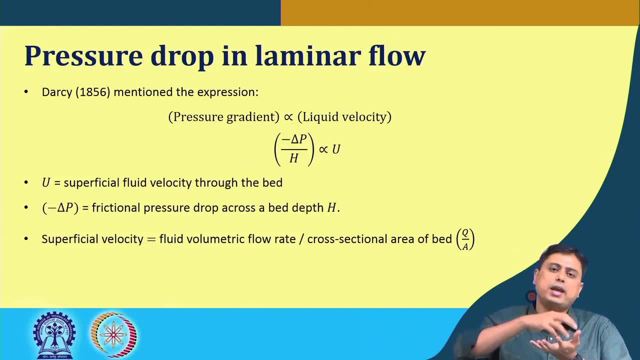 That you, let us say you take a beaker, you put some sand inside. ok, Now the sand will fill some portion, what the some height of this beaker? ok, but there will be some void spaces. ok, So if you pour some water, that water can be soaked in that void spaces, or 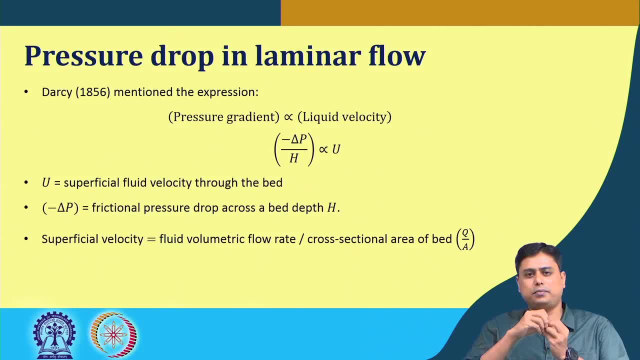 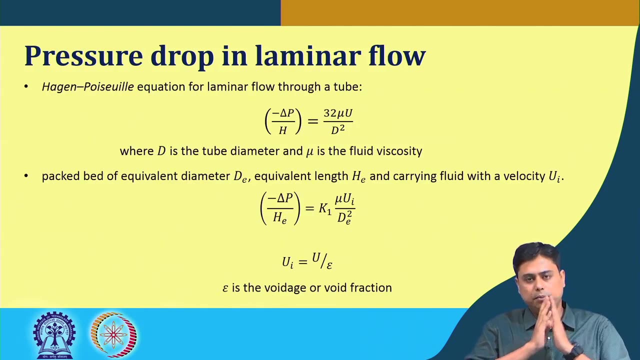 the empty spaces in between the sand particles, Now that space we call as the void space or the voidage. ok, So the point is, when we talk about such bed of particles, then to understand the pressure drop across such bed. ok, Initially, let us 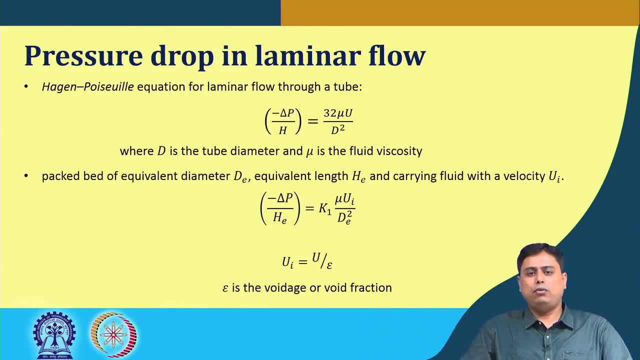 start with the pressure drop of a laminar flow through a tube. We already know that expression, the derivation part. we will not go into detail because this is the part where the prerequisite fluid mechanics knowledge will come into play. So this Hagen Poiseul. 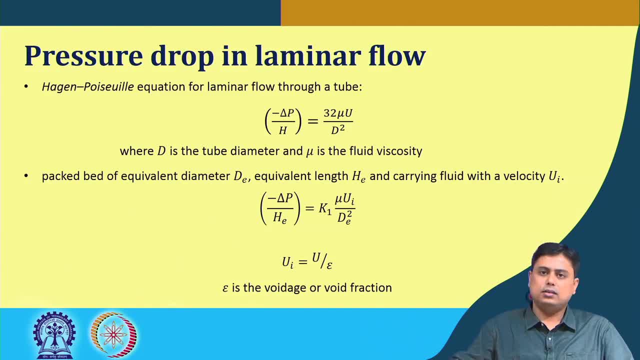 equation for laminar flow through a tube has such expression that you can remember or recollect this expression, Ok, where D is the tube diameter or the pipe diameter and mu is the fluid viscosity rest. other parameter: we have already defined that this is the pressure gradient per unit length or per unit depth. 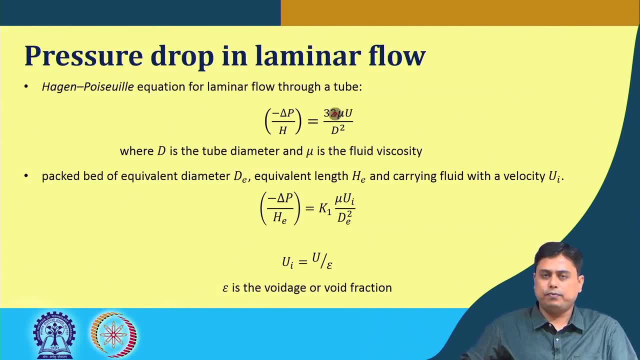 of the bed. U is the superficial velocity. The point here is that the packed bed or a stack of particles of a certain height, of this H again- can be thought of if, let us say, somehow you have managed to fill the beaker with a known size: spherical particles in a 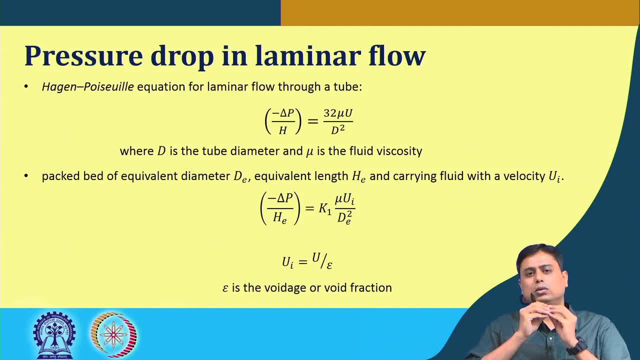 sequential manner, Then it is possible to imagine that the void spaces in between the particles are of this kind of a density: The tube shape, void space, ok, So, which means the void spaces inside the packed bed or the stack of the material. can be thought of this: several tubes that are 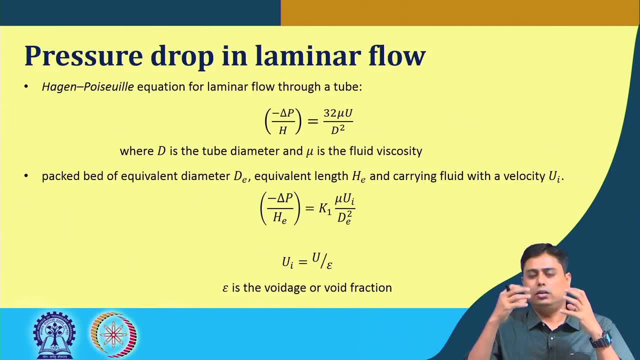 there, inside the bed through which the flow can happen, and if that imagination you can do equivalent diameter d e with the equivalent height h e, that carrying a fluid that is of velocity, u i ok, This u i, we say the local velocity or the interstitial velocity, interstitial. 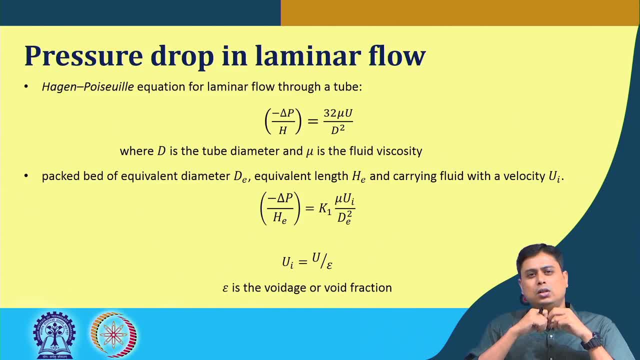 in between the particles, ok. or the local velocity: ok. Then the similar expression we can write for this packed bed as well. that is, minus del p by h, e, which is the equivalent height- ok, considering those many of tubes that are there- The superficial velocity of u, the interstitial velocity, that is u, i and the equivalent diameter. 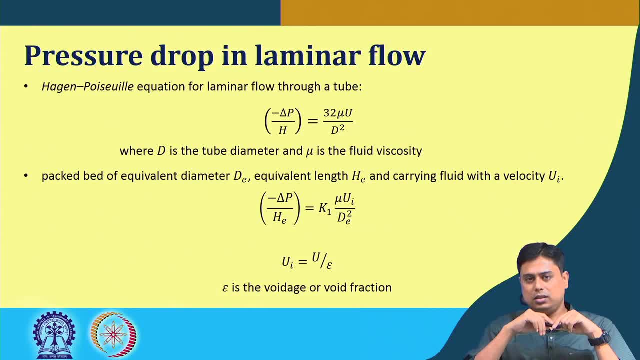 d, e, where k is a constant. ok, that depends on the shape of this tubes path, because the tubes path are basically not straight. ok, So the point is that it will have tortuous path in reality, through which the water or any fluid can flow when there is a stack of. 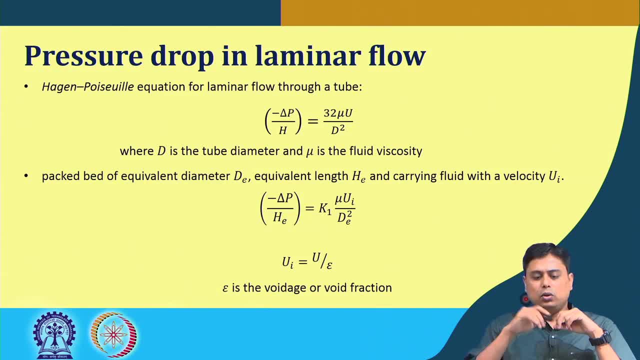 particle. ok, So this interstitial velocity is nothing, but it is the superficial velocity divided by the voidage or the void fraction that is available for the flow. This voidage, again let me define that it is the empty space in the bed divided by the total volume of the 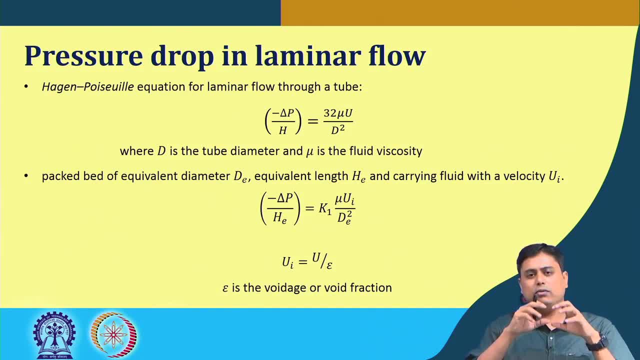 bed. It is a dimensionless number. it quantifies that. how much available space is there for the flow? ok, So when we divide the superficial velocity with this value, then we can have the interstitial of the local velocity. Quite naturally, this local velocity is always higher than the superficial. 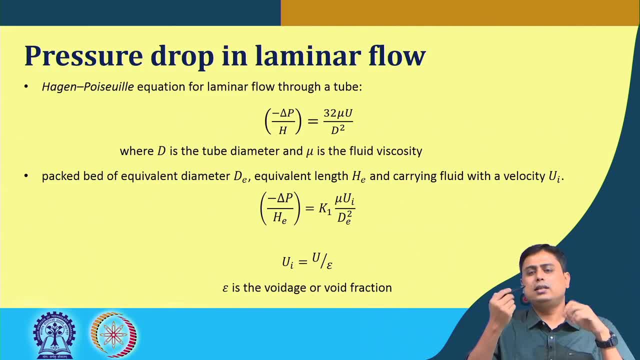 velocity. So the superficial velocity is something like that. what you poor in that beaker? ok, that comes from the volumetric flow rate divided by the cross sectional area of the beaker, And then in the water when it flows inside those sand particles, those velocity, if you. 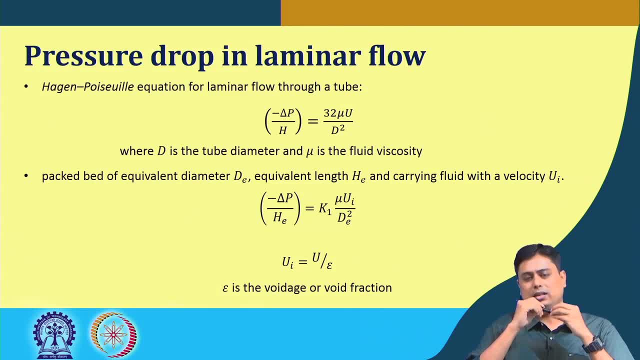 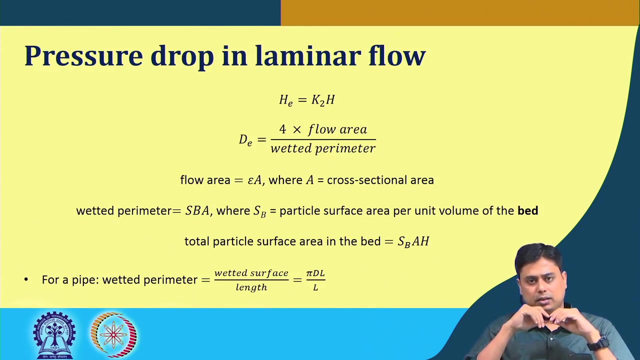 can measure, that is the local velocity or the interstitial velocity And that is the superficial velocity divided by that voidage or the voids space that is quantified by this epsilon value. ok, So the relation between interstitial velocity and the superficial velocity should be clear. Now, as I said, this tortuous path in the bed. 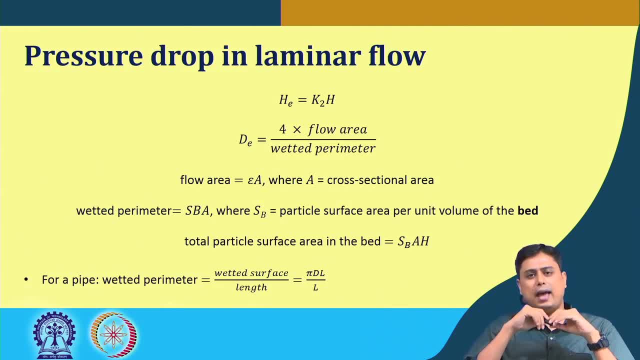 ok. or through the interstitial where the flow is happening, can be thought of as a proportional value to the bed depth. As the bed depth or the height increases, this tortuous path naturally increases. So this equivalence to the horizontal velocity and height is basically factor is of the total height. ok, And that proportionality constant. 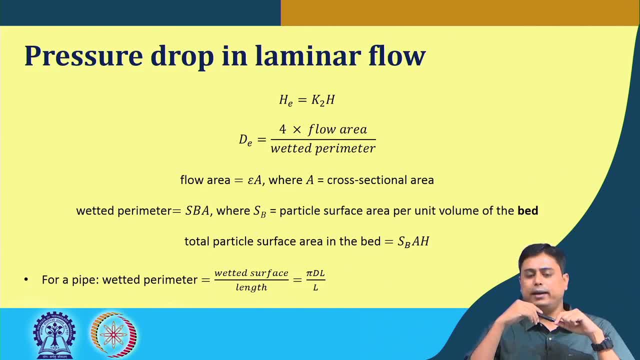 is here k 2, where the h is the total bed height, The equivalent diameter or the hydraulic diameter. how do we define It? is 4 multiplied by the flow area divided by the weighted perimeter. So weighted cross section by the weighted perimeter. ok, 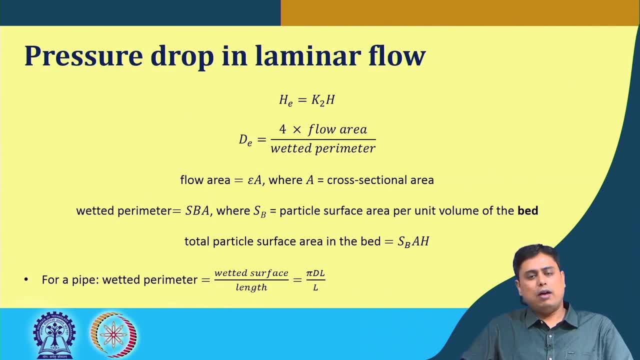 Now here, if you have understood the concept of voidage, now that voidage is through which the flow is happening. So if A is the total cross sectional area, actual cross sectional area, the area available for flow is basically epsilon multiplied by A, because other portions 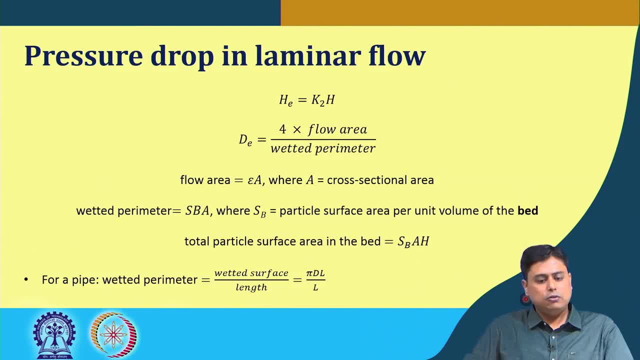 are filled by the solid particles. So this flow area is then epsilon A. the weighted perimeter is at the S superscript B. This B would come at the bottom due to something here that is not showing properly. but it is actually S B at the superscript light. it is written here. So if that is the 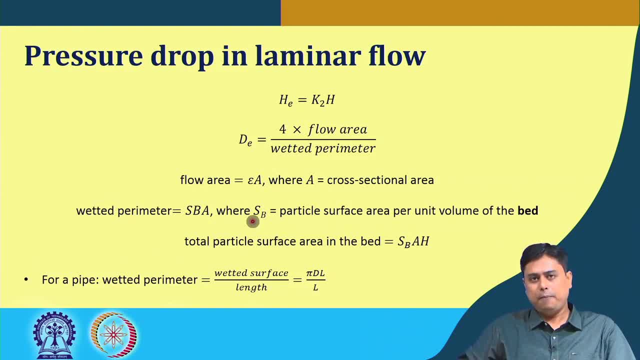 surface area per unit length, then if I set this So for this situation, that will give per unit volume of the bed. ok. then the weighted perimeter is basically that multiplied by the cross sectional area, Again S, b, if we define that, the particle surface area per. 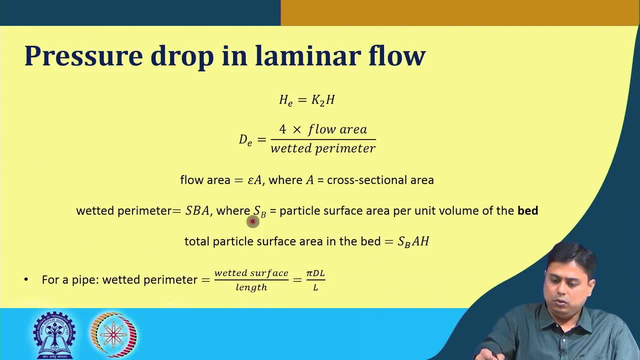 unit volume of the bed. ok, So this is the per this quantity. if we define on quantity as a particle surface area per unit volume of the bed, then the weighted perimeter would be this particle surface area per unit volume of the bed multiplied by the cross sectional. 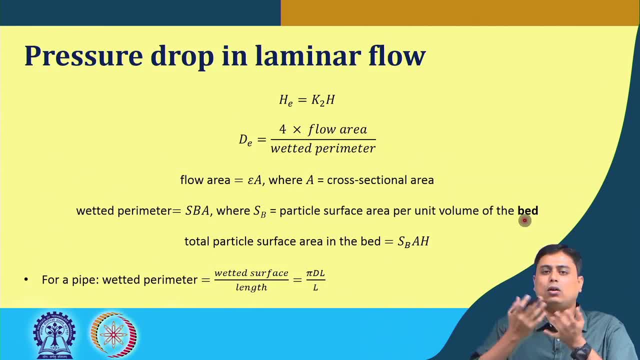 area, That is what the water or fluid can weight. that is that much area of the particle, of the particles. ok, So the total particle surface area in the bed, then this area, this quantity multiplied by this h, that is the depth or the height of the bed. 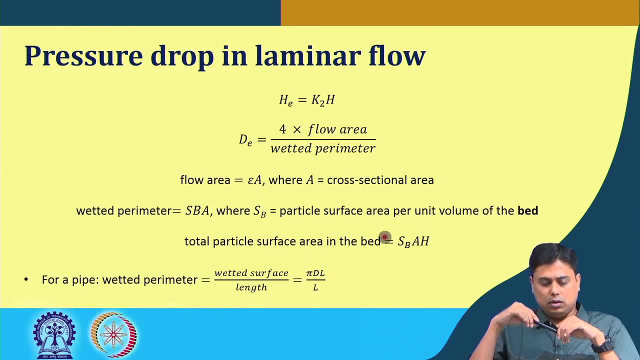 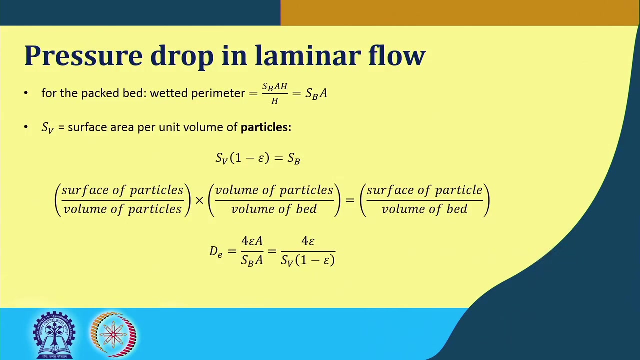 So now, in other way you can think of this: for a pipe, the weighted perimeter is the weighted surface by the length, which is pi by L. ok, For packed bed, the weighted perimeter analogous to that ok will be of one 값, Sb A, H divided by the length of the packed bed, and that gives that Sb multiplied by the. 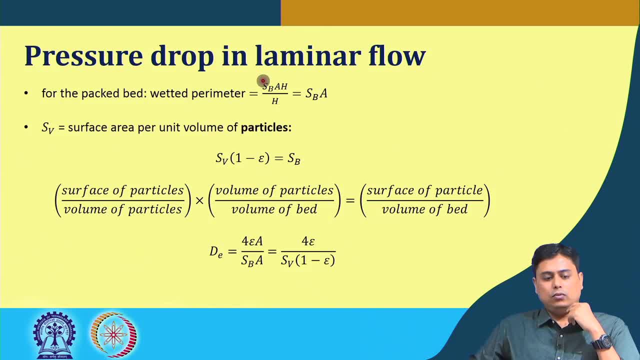 A value. So this would be our weighted perimeter. Now, if we define another quantity, is that surface area per unit volume of the particles? ok, the surface area per unit volume of the particles, Sv, then Sv multiplied by 1 minus epsilon. 1 minus epsilon is basically the solid. 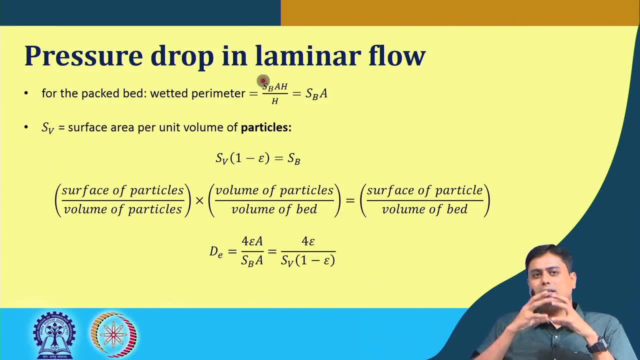 quantity multiplied by the surface area per unit volume of the particles is basically the surface of the particles per unit volume 횩 diligent wh volume of the bed. So in a more simplified manner, if you follow this expression, that surface of particles by the volume of particles, which is basically 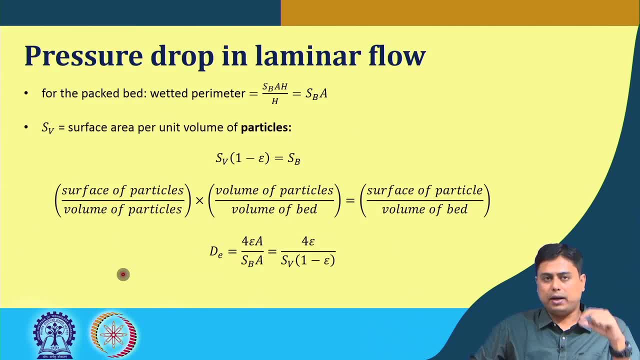 the S d surface area of particles per unit volume of the particle multiplied by volume of particle per unit volume of the bed, which is nothing but 1 minus epsilon, because epsilon is volume of empty space divided by volume of bed. So 1 minus epsilon is the volume 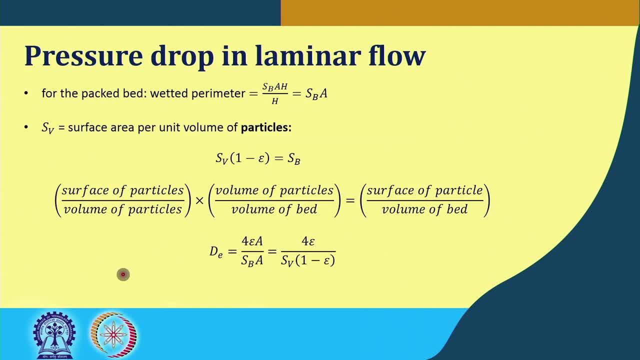 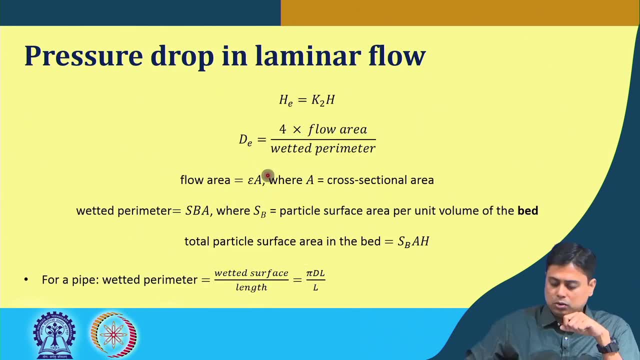 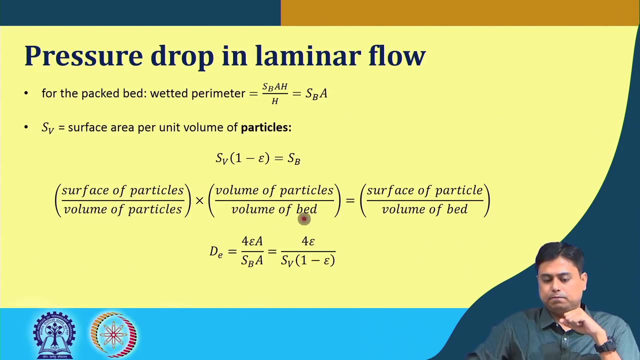 of particle divided by the volume of bed, and that, eventually, is this denominator. denominator goes out, So it becomes surface of particles, Surface of particles per unit volume of the bed, which is nothing but S b that we defined earlier. ok, The reason we are doing this is to calculate the equivalent diameter or the 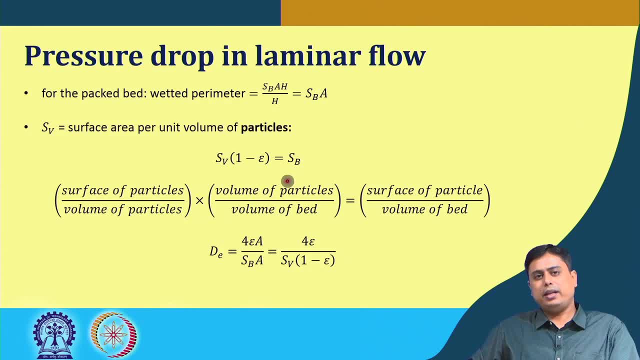 hydraulic diameter. Now hydraulic diameter. again. we go back to that expression, previous expression, that is, 4 multiplied by the weighted cross section, divided by the weighted perimeter. So 4 multiplied by the weighted cross section is epsilon a multiplied by a. epsilon multiplied by a divided by this S b a, where S b is nothing but S v, multiplied by 1 minus epsilon, The. 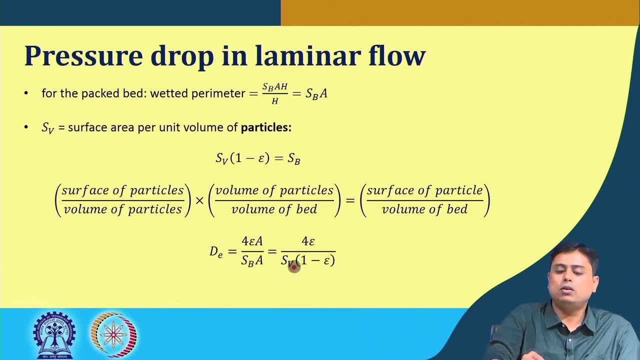 reason we have converted the S b to S v, because S v is the particle area, It is a particle, particle property. now, For any particle property, any type of particular shape, you can find out what is the S v value. ok, So for spherical object, this S v is what S v is, nothing but. 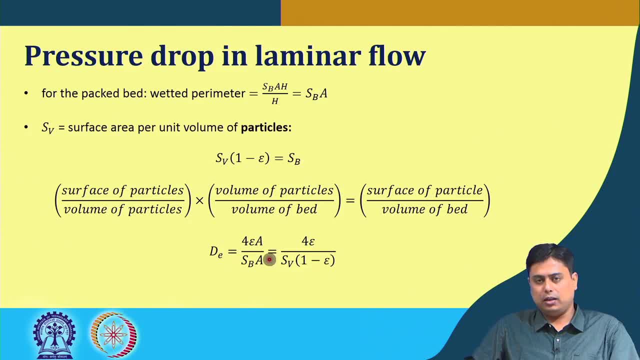 6 by x or the diameter of the spherical object. It is the surface area of the particle, that is the pi d square, ok, and the pi d cube by 6 at the denominator, that is the volume of the particle. So that is why we have converted that, because 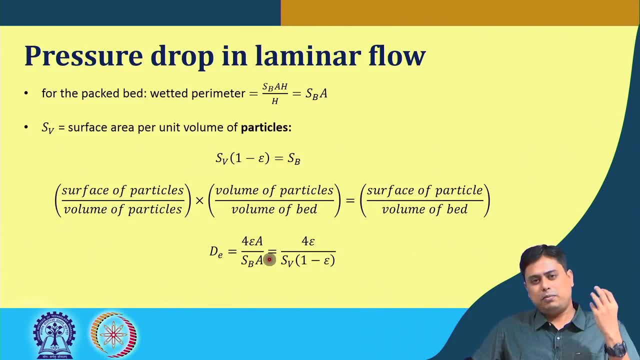 we are finding out the generic expression ok, irrespective of whatever the particle shape is, so that we can understand how much will be the pressure drop across that bed of different types of particle. different that shape can be of different type. So, having said that, so, which means the d e, we get as this expression the equivalent. 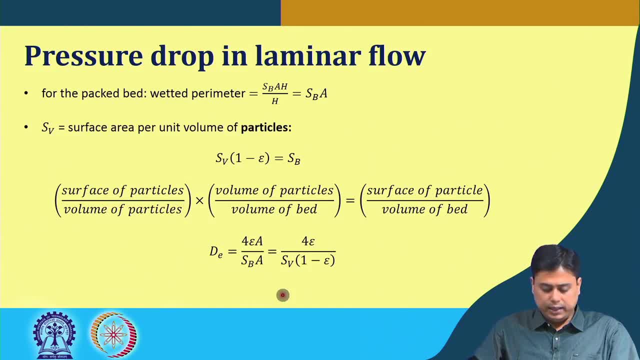 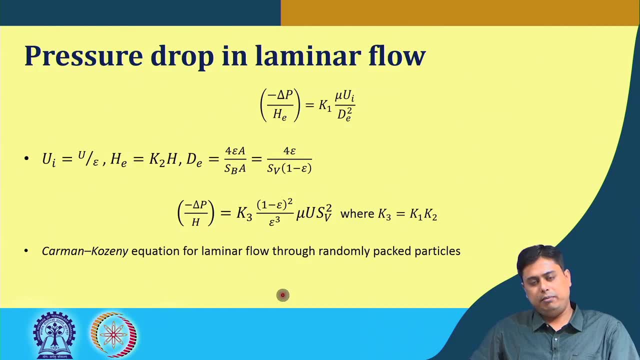 diameter. and then what we do? We go back to this expression that del p by h e was a constant multiplied by mu Mu, u by d e square. ok, So here now we replace all these equivalent terms where u i interstitial velocity, which is difficult to measure. So let us convert that to the superficial velocity. 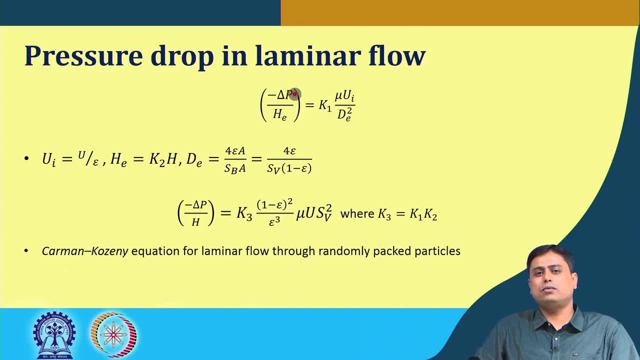 which is easier to measure because this we directly get from the input values or the inflow rate. So that is superficial velocity divided by the void space. Equivalent height is a constant term multiplied by the height of the bed, because again, the equivalent height is not the straight. 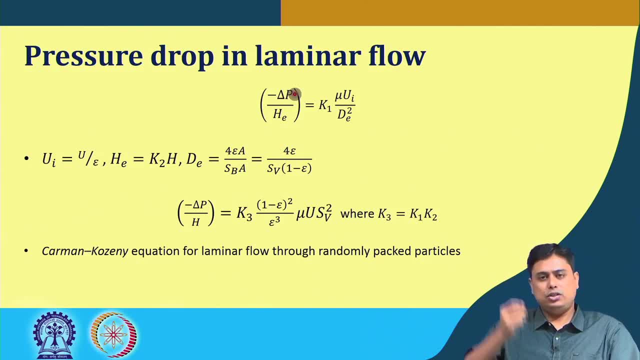 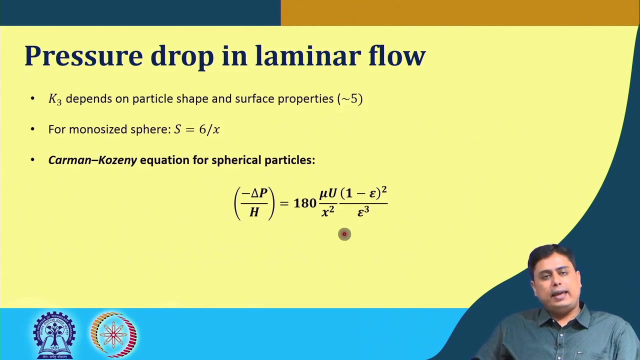 height. in case of tube it is just h, but here it is a tortuous path through which the flow is happening. The constant term depends on the particle shape and surface properties. it has been observed by several experiments: a wide range with a wide range of particles, wide range of particle types having different density, different shape. 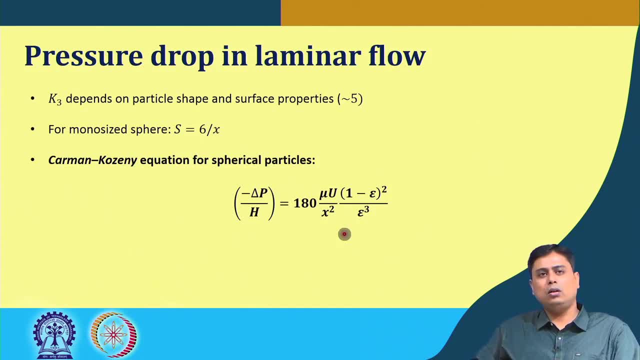 It has been seen that this K 3 value depends on the particle shape and surface property, and this value is numerically close to 5. It has been a constant value of 5.. Now for monosized sphere, monosized means. 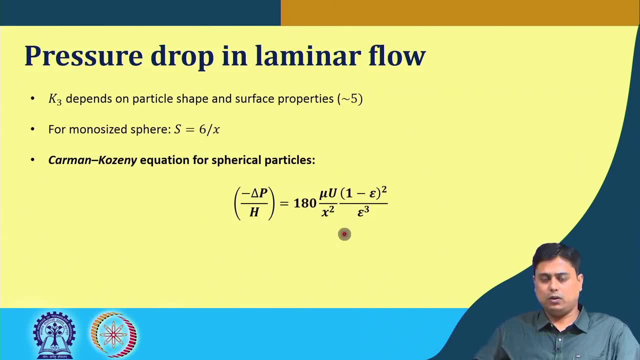 the sphere of same size, of same diameter, let us say x, all the spheres. ok, So in that case, if you make a packed bed of those spheres of diameter x, of height h, then the del P across that packed bed will be this expression. because if we now put K, 3 value as 5 and S, 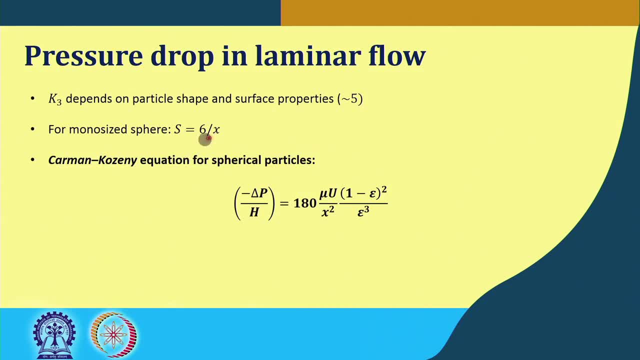 V that was there. S V square is 6 by x, We get 180.. So 180 multiplied by this factor, mu u 1 minus epsilon square, by epsilon cube divided by the x square that is already there, This is again a famous form of the Kozeny Karman equation. 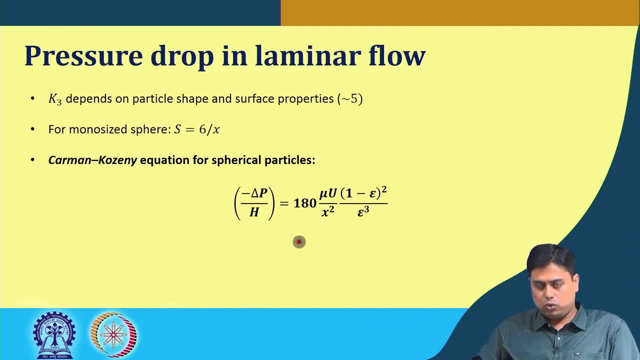 for spherical object, again: monosphere. spherical object: laminar flow. These conditions have to make be met. then you can use this expression to find out what would be the pressure gradient across a spherical mono sized spherical object of diameter x When a fluid of viscosity mu. 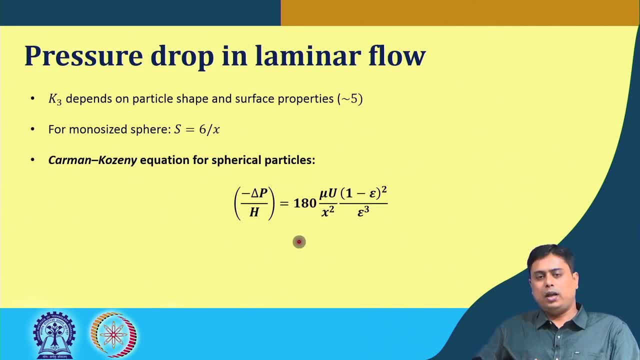 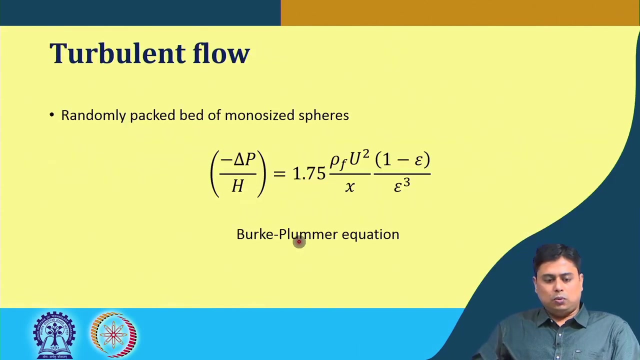 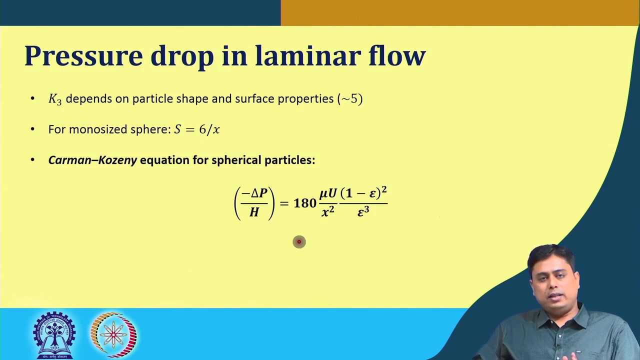 is flowing at a superficial velocity of u and when the bed void is epsilon. that is known to you. If this criteria or this information you have handy, then you can use this formula to calculate this pressure gradient or the pressure drop across the bed. So this is the laminar condition. ok, When there is a flow through the packed bed of 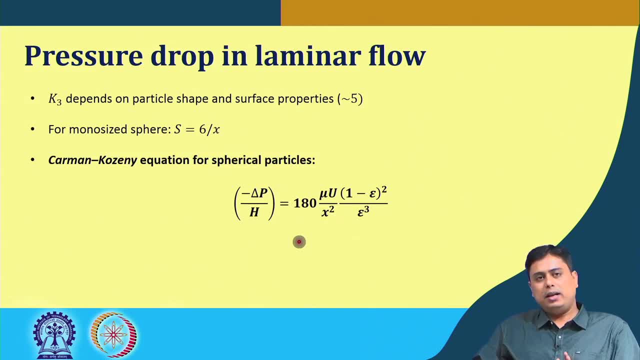 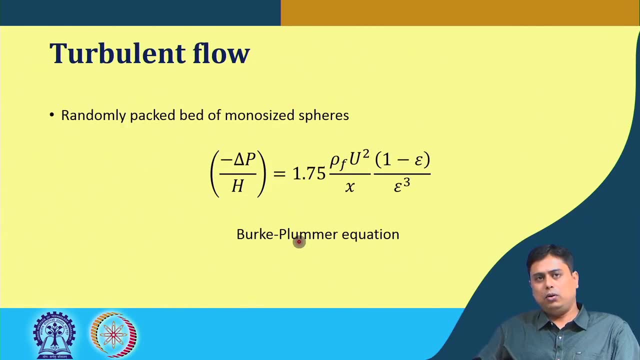 a mono sized sphere. So, similarly, what could have been the pressure drop for the turbulent flow? For the turbulent flow in a randomly packed bed of mono sized sphere, the expression is this: one which is minus del p by h, here we have 1.75 as the coefficient. rho f? u square.